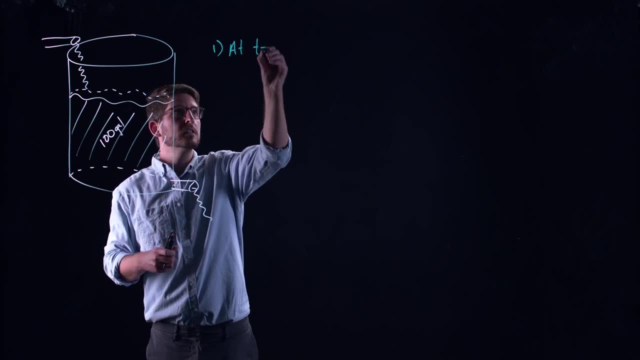 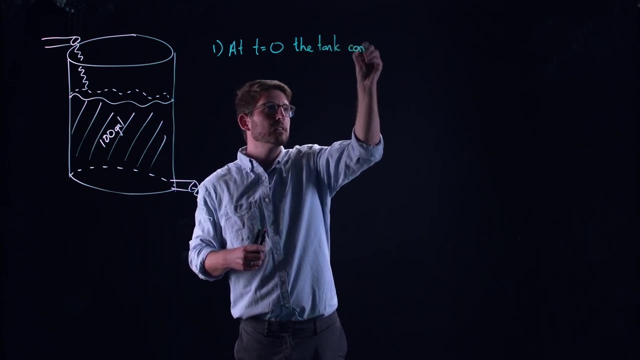 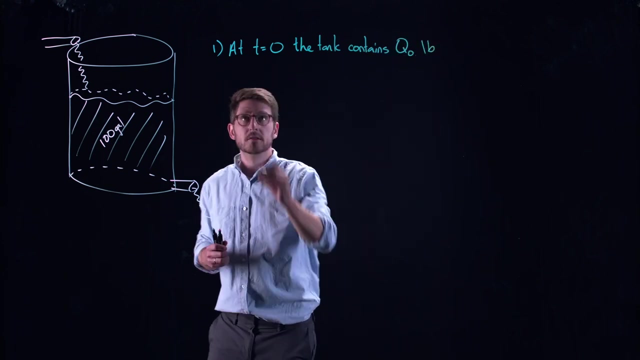 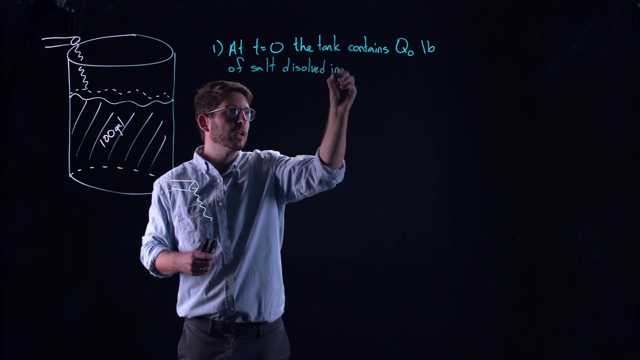 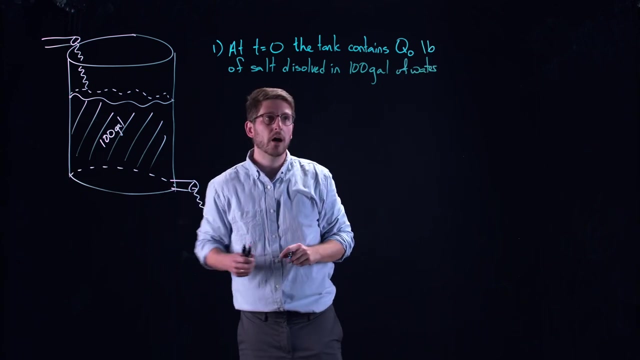 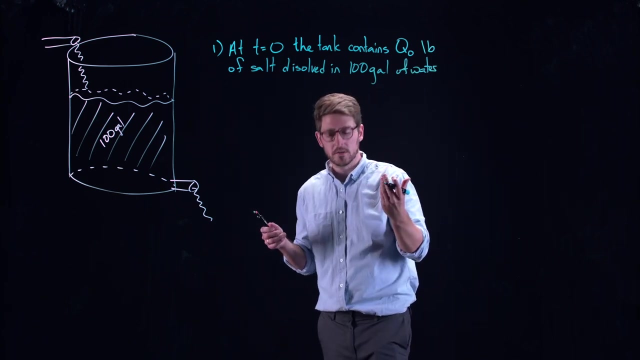 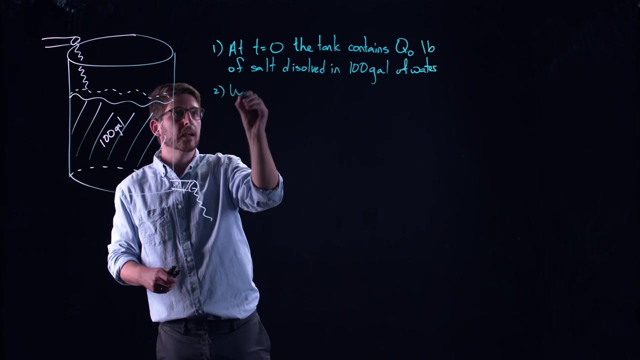 So the first thing is that at time zero, the tank contains- let's call it, q, naught pounds lb of salt dissolved in a hundred gallons of water. Okay, so inside of that tank there's a hundred gallons of water with q zero or q naught pounds of salt that's dissolved into it. Okay, now, second piece here: water containing. 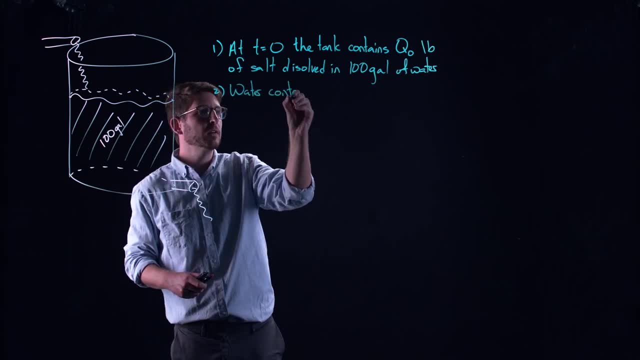 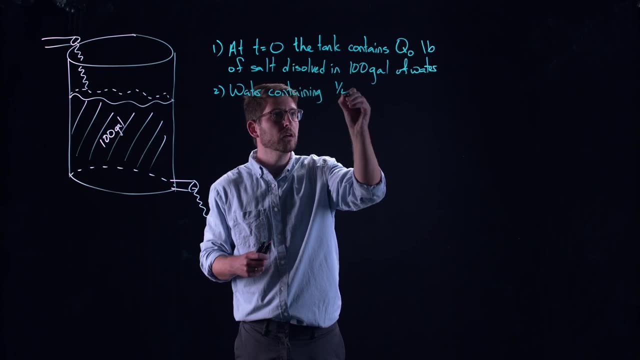 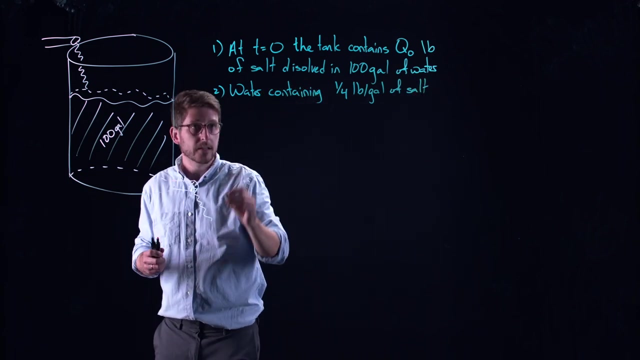 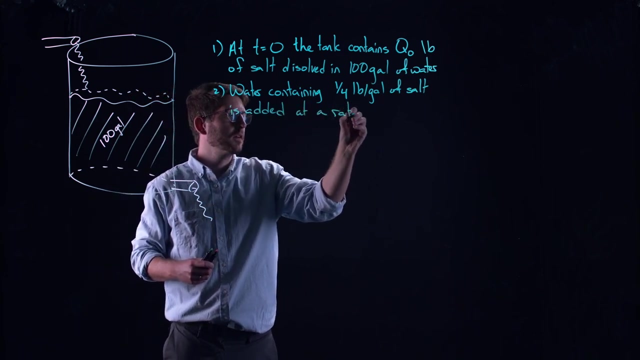 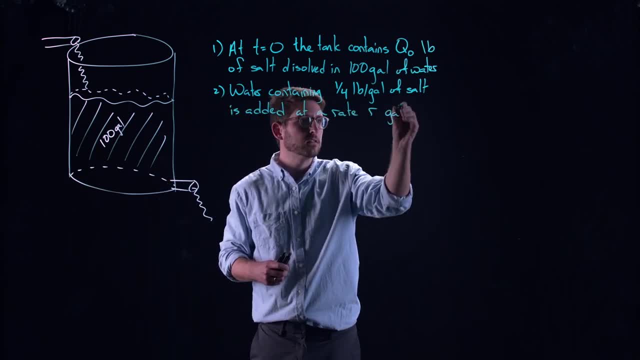 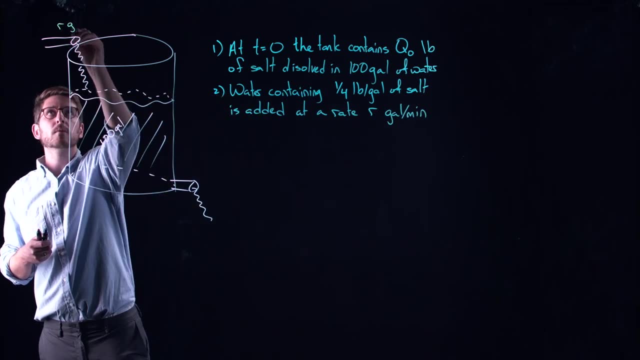 effect, or somebody that you know leaves you out of this question. so again, a break up of the rules. this is just in case you don't want to, because we're not gonna hit ourselves a lot easily with this kind of stuff. So the first thing that I'm gonna put in there is that salt contains one and a half. 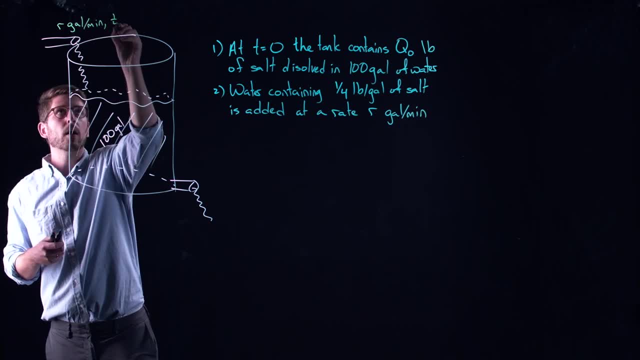 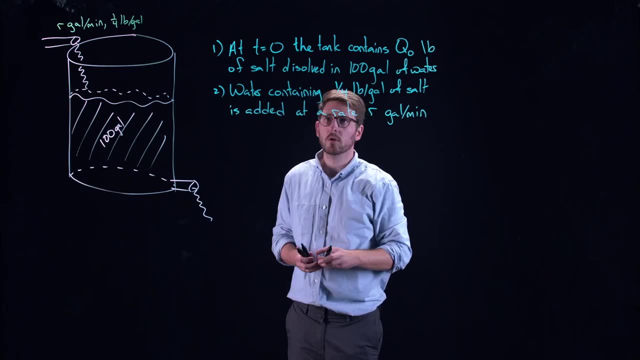 pounds per gallon of salt. checking out the table: Okay, so let's go right over here now. So this answer- Fucked, Okay, I'll put in right here. So this goes down here. so these will be Sounds good, and it's got one quarter pounds per gallon of salt. Okay, so that's one more piece that we can. 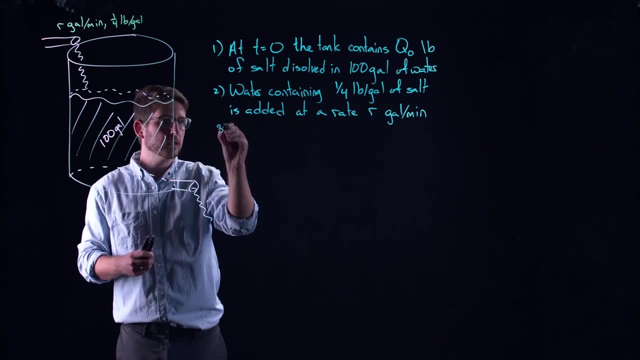 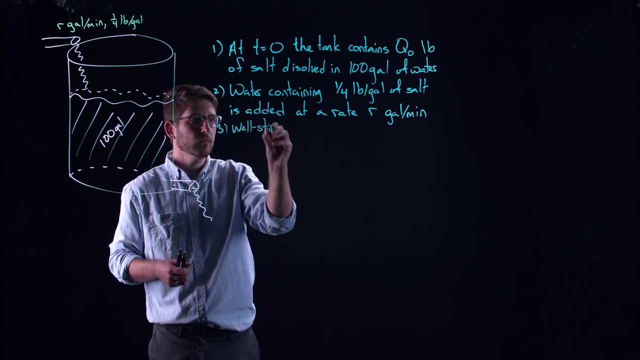 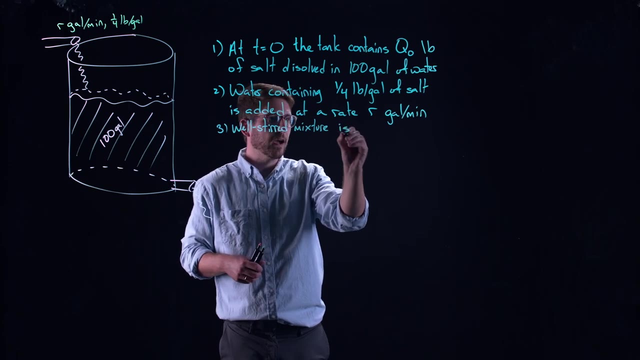 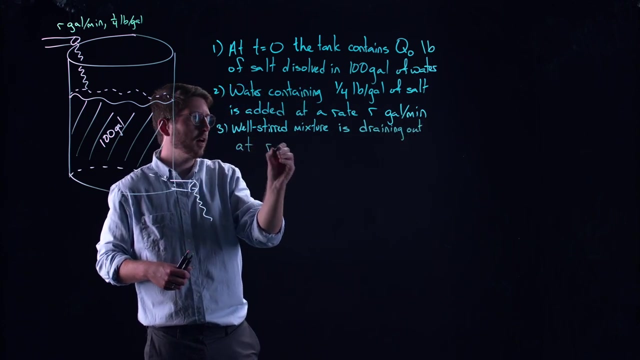 fill into this, and the third thing that we can say about this is about the water going out. So there's a well stirred mixture- so I'll explain that in a moment- and it's draining out at the same rate, at our gallons per minute. Okay, so that means that water is coming out of this. 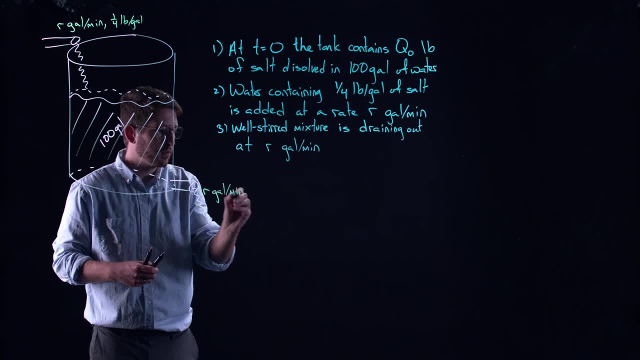 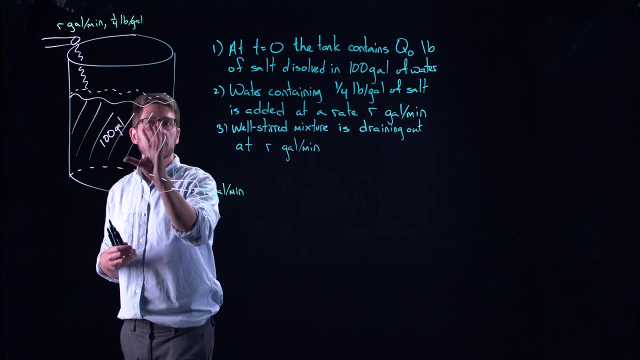 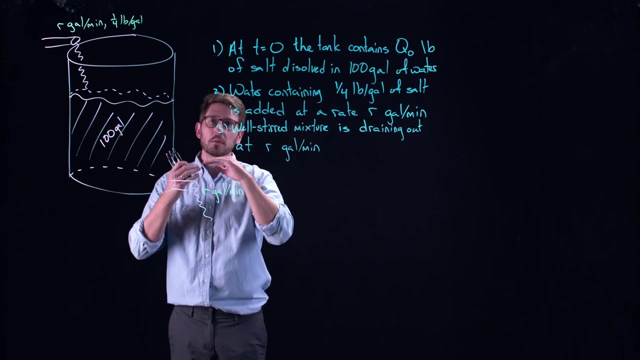 spout similarly at our gallons per minute. Okay, now what does it mean to be well stirred? That means there's something going on- maybe a little turbine or something like that- inside of the tank that is mixing up the salt so that we have a completely uniform distribution. So if you 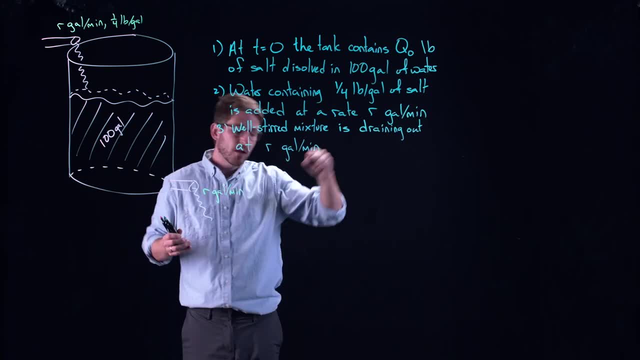 dip a spoon in the salt and you pour it into the water, you're going to have a well stirred mixture. So if you dip a spoon in the salt and you pour it into the water, you're going to have a well stirred mixture. So if you dip a cup in and you take out some of that salt water and I dip a cup in and also 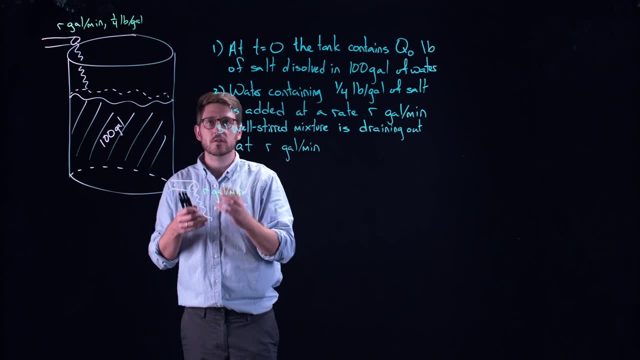 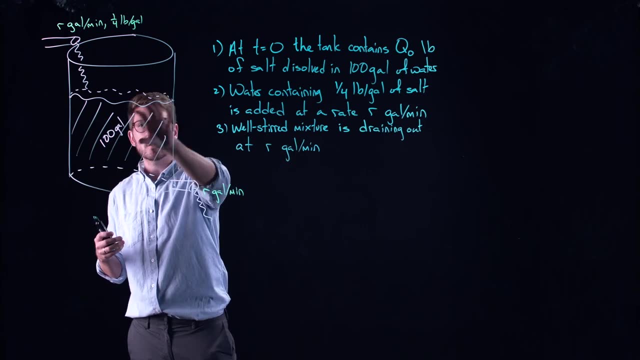 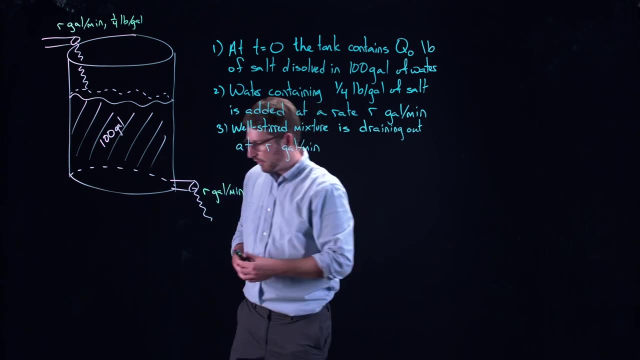 dip out some of that salt water, it's going to have the same amount of salt per gallon in it, All right, so it's mixed up in such a way there's not regions that are also, or a lot more salt here and less salt there. Okay, we're assuming a uniform mixing of the salt, All right. so how do we do this? 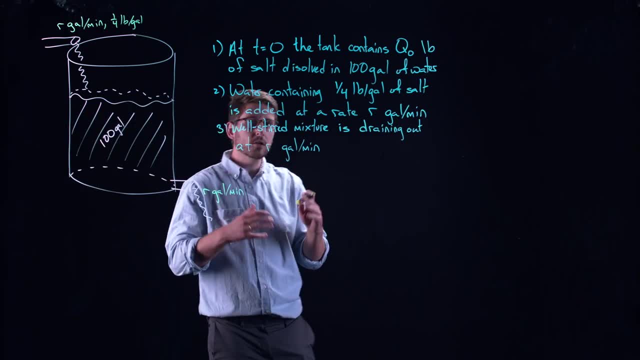 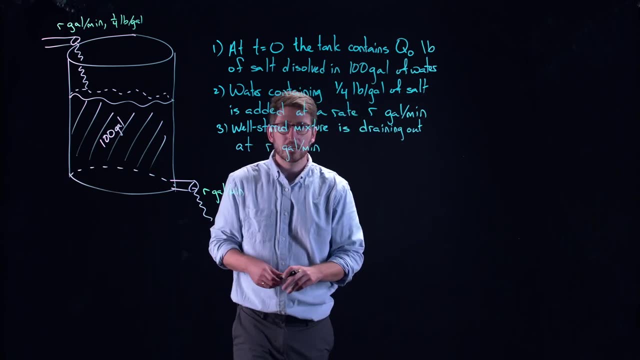 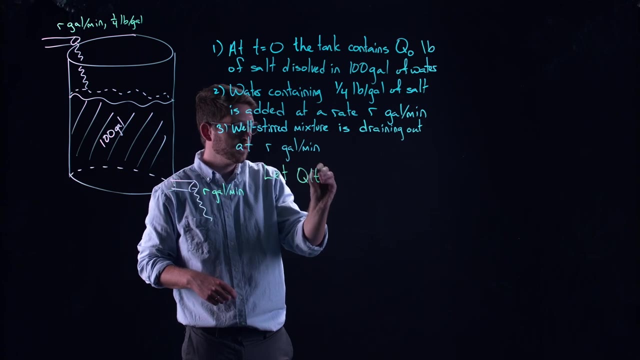 How do we approach this problem? Well, what we want to do is we want to set up a differential equation, And that differential equation is going to be for the amount of salt inside of the tank. So let's say, let q of t be the amount of salt. 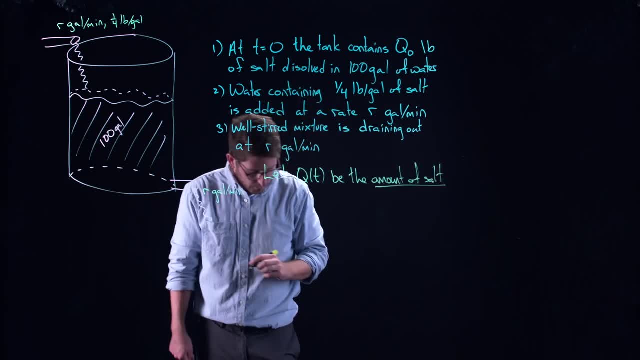 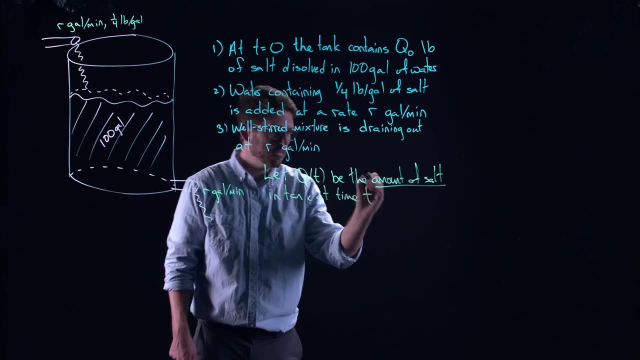 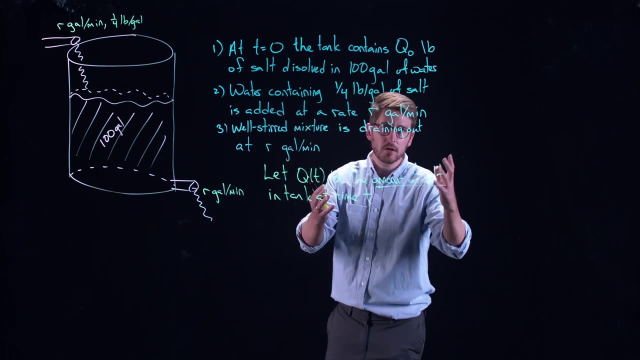 so the amount of salt, uh in the tank, so in the tank at time t. okay, Now what we would like to do is we'd like to set up an initial value problem. Now remember, initial value problem is composed of two different components. First of all, the problem component. 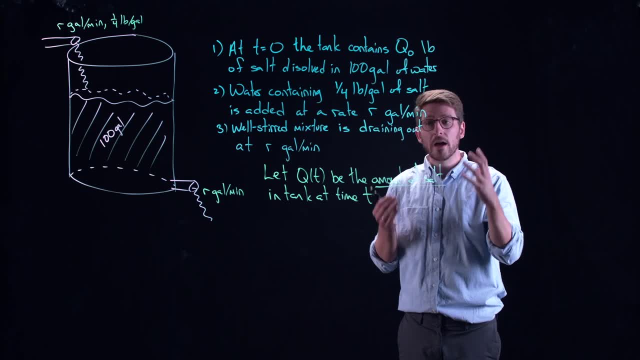 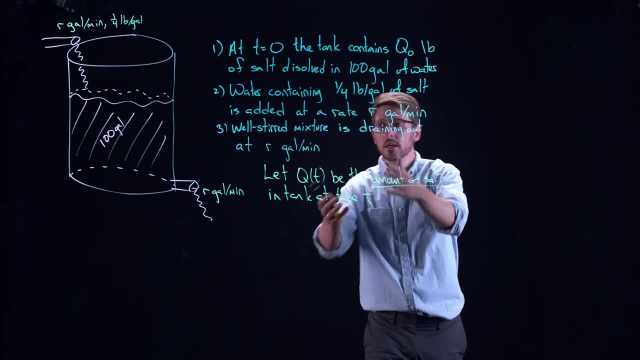 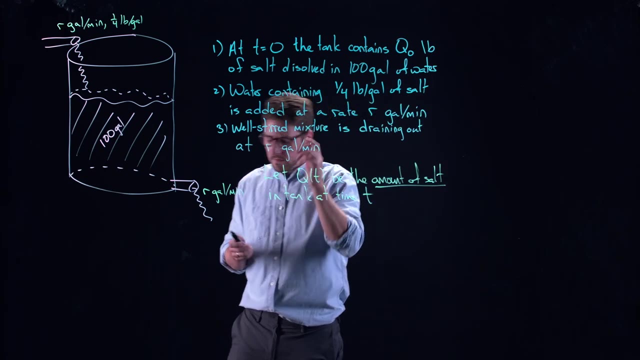 that's the differential equation and the initial value component, And luckily for us, we already know the initial value. It's right here. So we know that q of zero is equal to q naught. That's good. That makes our life slightly easier. The question is: how do we set up? 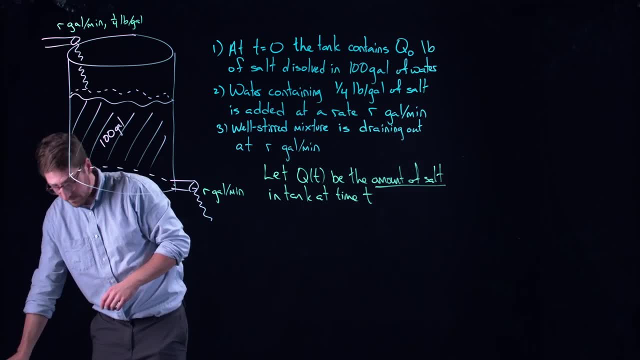 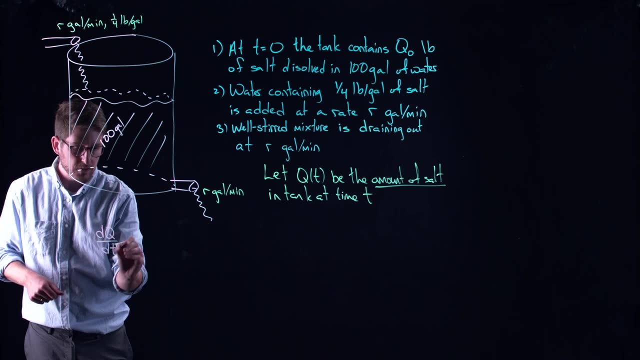 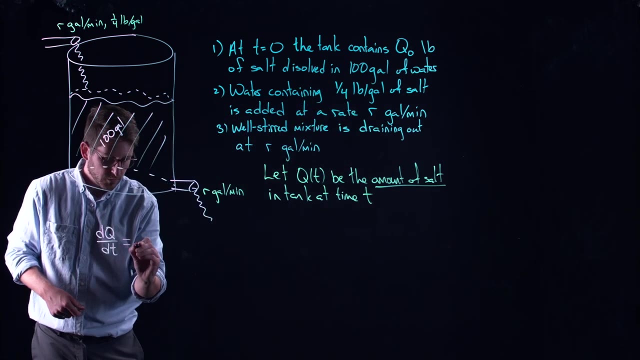 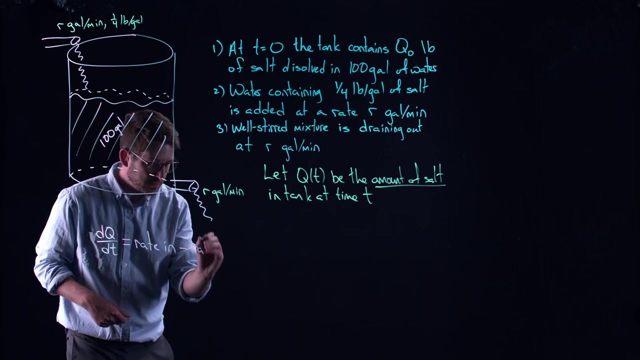 our differential equation that's going to be associated to this thing. Well, here is what we know: The rate of change of the amount of salt. okay, so the rate of change of the amount of salt is going to be the rate at which salt is coming in to this bucket, minus the rate at which salt is going out. 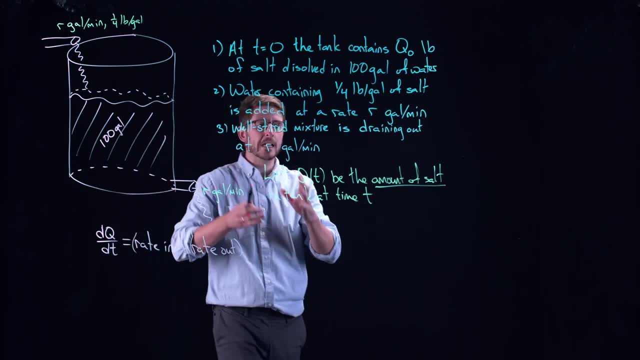 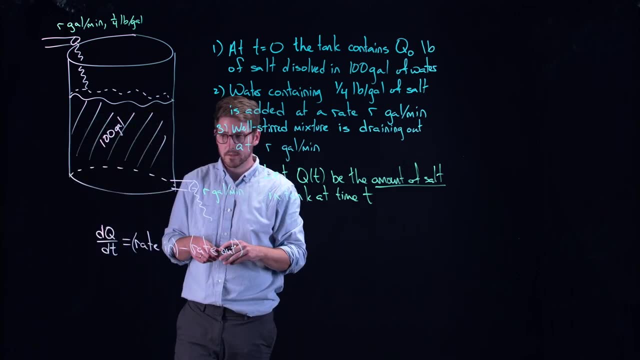 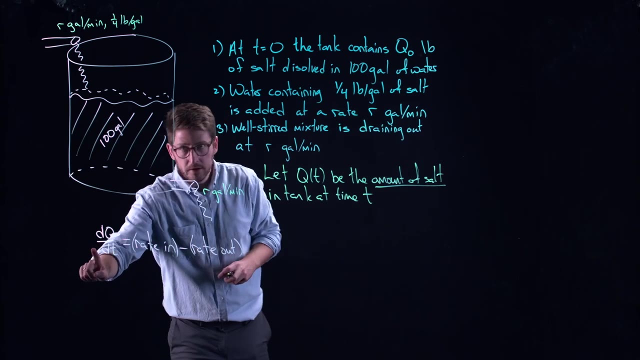 Okay, let's do a little bit of unit analysis first, because this is the best way to figure out if we are in on the right track when we're trying to analyze this thing. q is the amount of salt in the tank. It's going to be measured in pounds. That means that the derivative, which is a rate of rate of 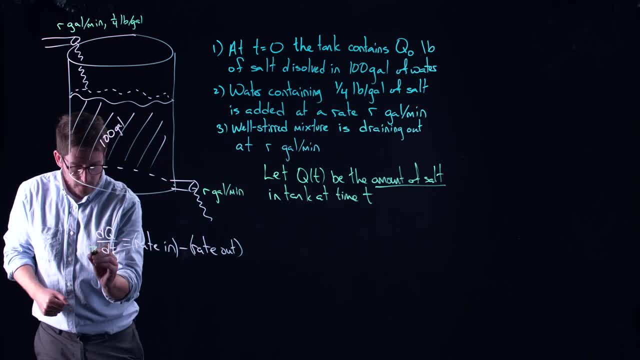 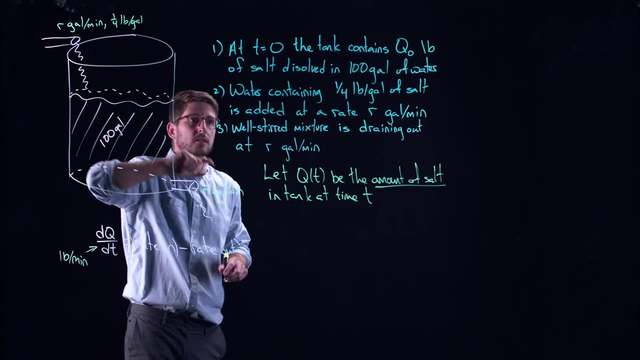 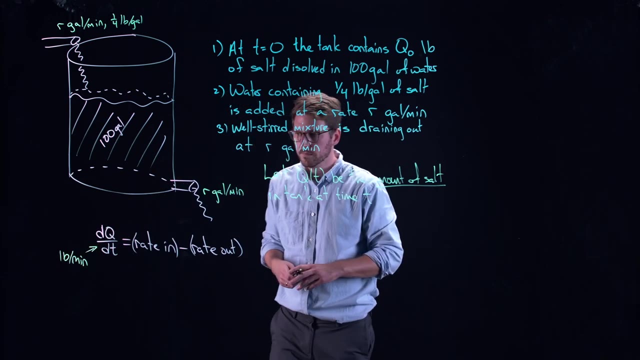 change. this thing is in pounds per minute. Right t is going to be measured in minutes. that's because we've been given a minimum. we've been given everything in terms of minutes. So the left hand side of this equation is in the units pounds per minute. That means that the right hand side also has to be in the units pounds per. 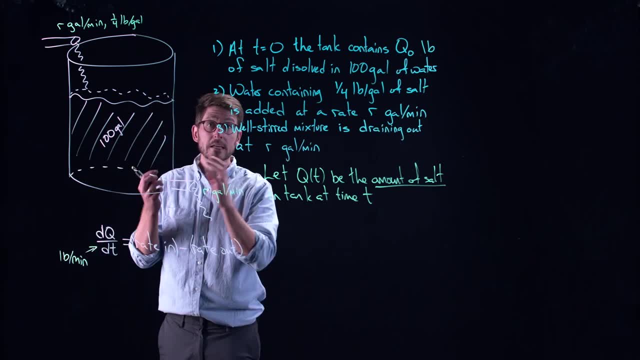 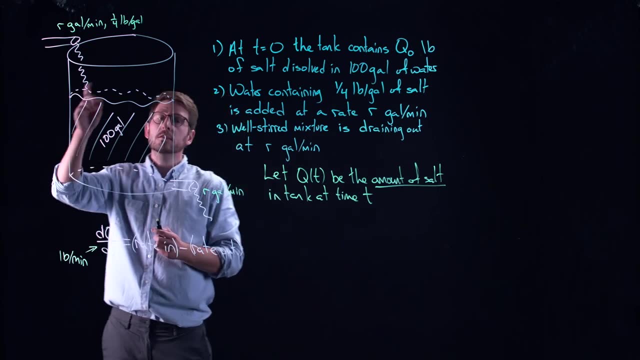 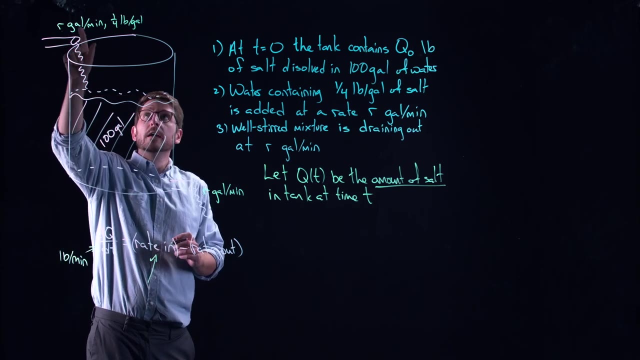 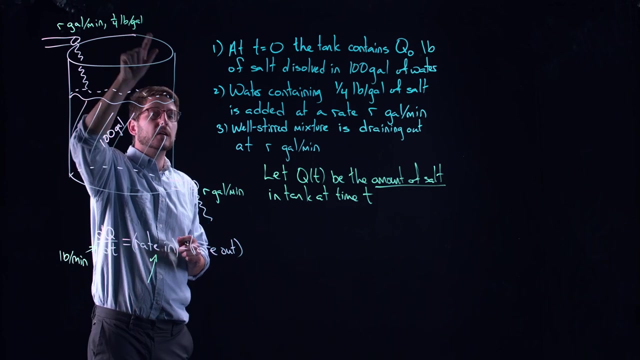 minute And, in particular, rate in and rate out independently have to be in terms of pounds per minute. Okay, let's just take a look at something. Okay, so for the rate in, we have our gallons per minute coming in And of those gallons that are coming in, we have one quarter pounds per gallon. 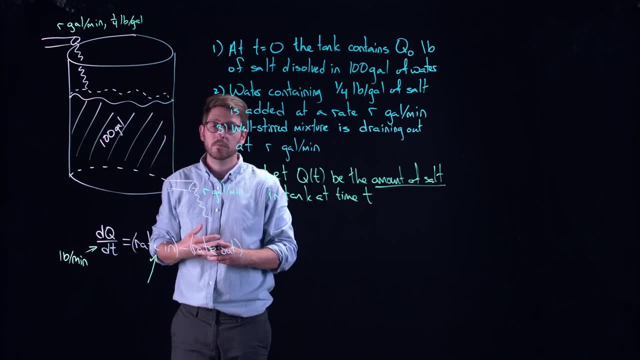 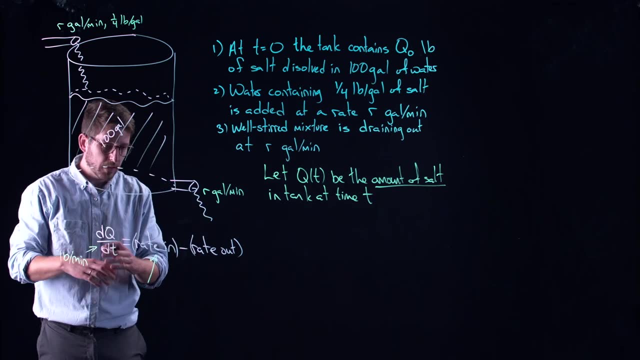 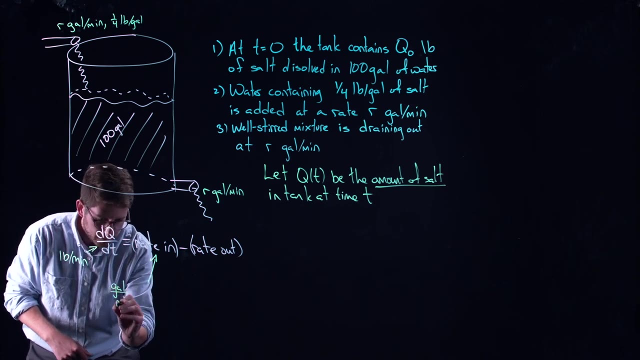 of that is salt. So what is the amount of salt that's coming in per minute? Well, let me just do. let's look at the units first, Just to analyze these fractions. So we have gallons per minute coming in And we have pounds per. 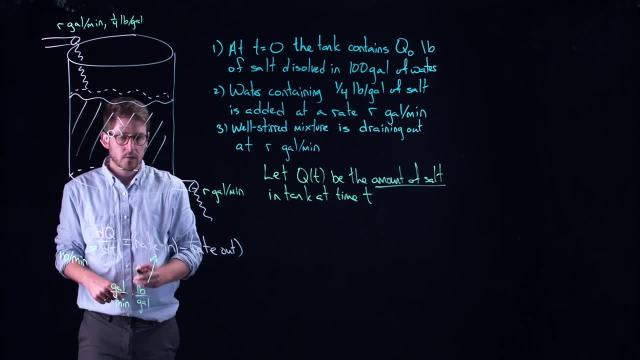 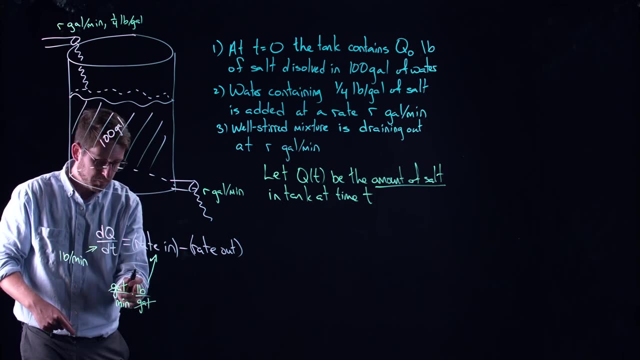 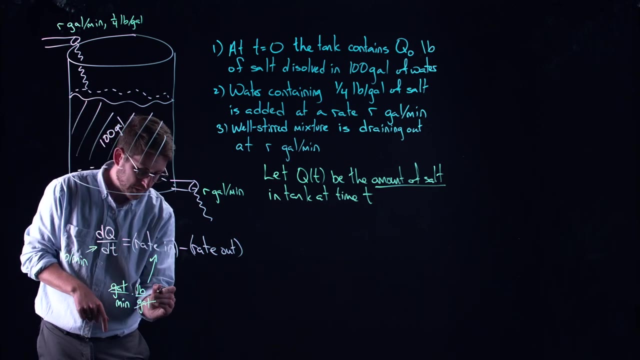 gallon of salt. That tells us that when we multiply these two things together, these things in these units, we get pounds per minute. Pounds per minute is exactly what we wanted, So that means that the rate in here is going to be in terms of pounds per minute, And that's exactly what we wanted. 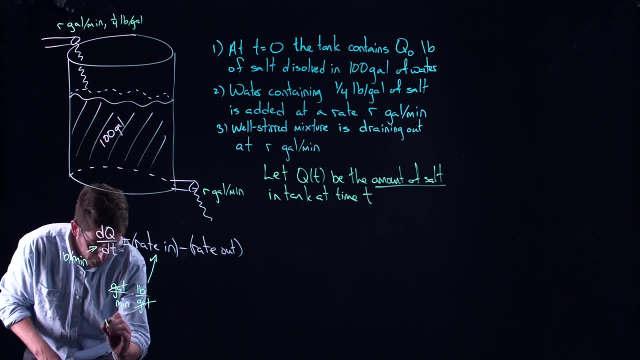 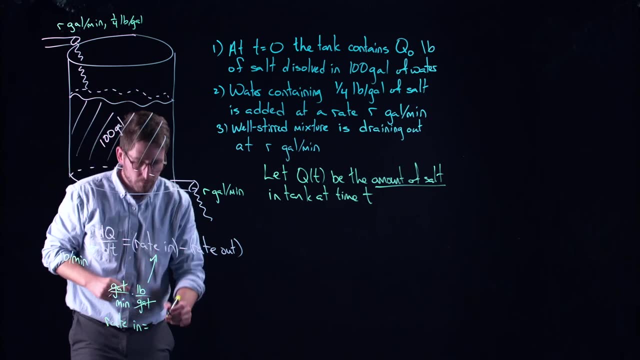 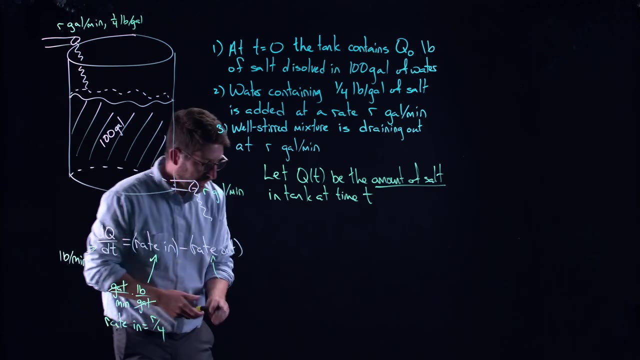 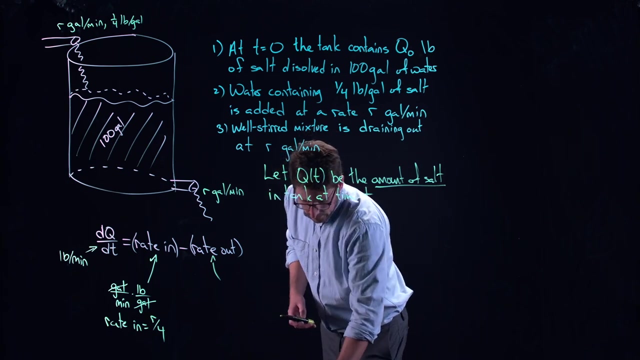 B. So rate in. Let's put it down here: Rate in is equal to multiplying these two things together: r over four. Okay, the rate out takes a little bit more thinking. Well, the first thing that we know about this is that we have the same rate of water coming in. 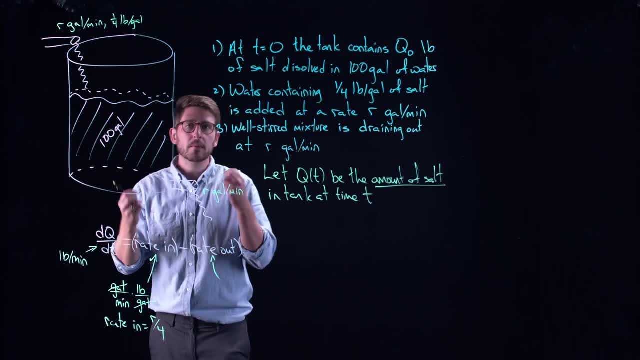 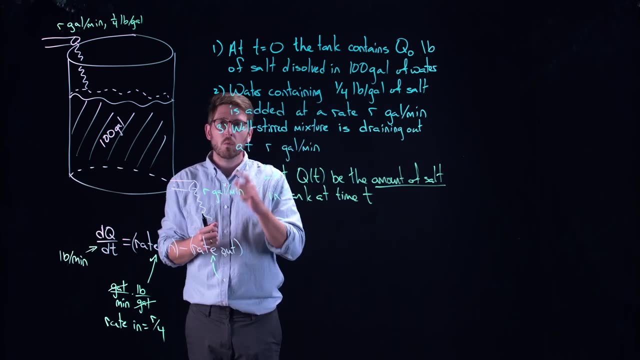 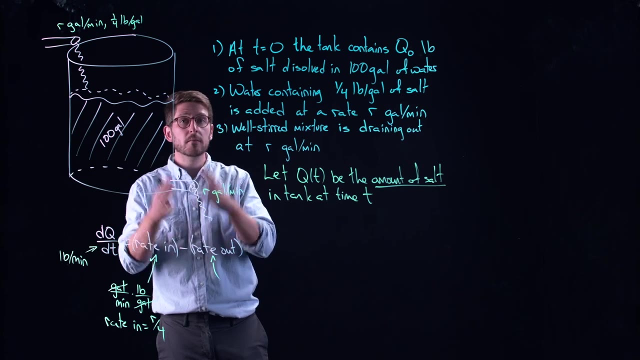 As we have going out. Now think about this in a different way. for a second Imagine: I've got a room full of people And I tell you, every single hour, one person leaves the room and one person enters the room. Well then, you would know that the number of people in the room never changes. The rate in 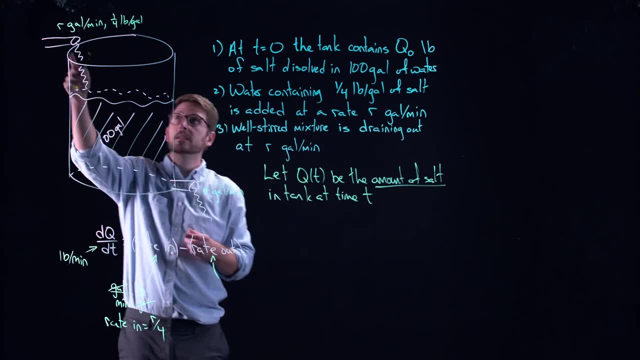 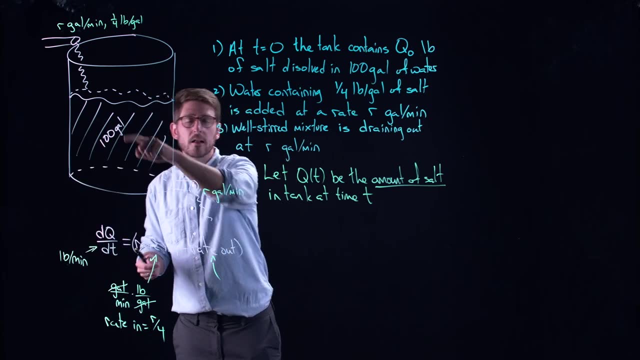 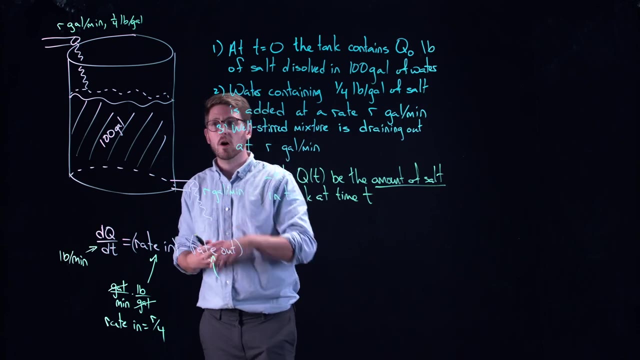 is equal to the rate out. Same thing is happening here. our gallons per minute is coming in. our gallons per minute is going out. You always have 100 gallons in this tank. You never lose the amount of water or you never gain an amount of water inside this tank. It's always 100 gallons. 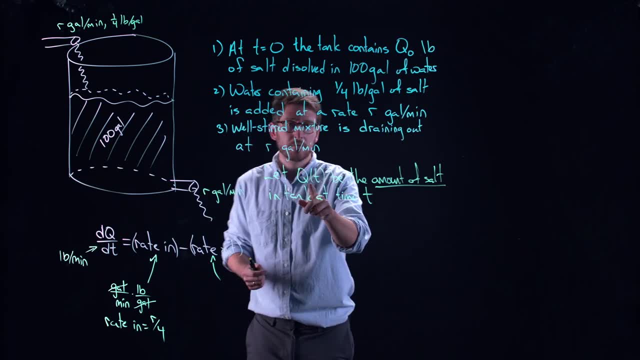 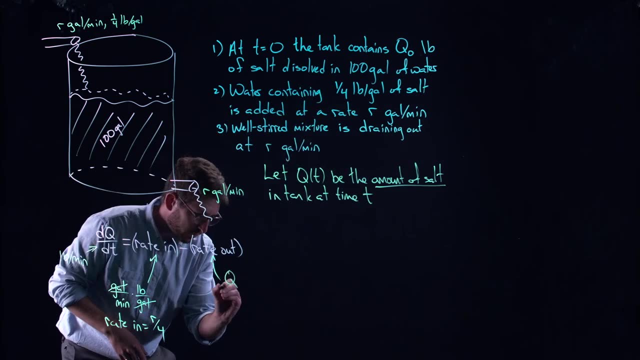 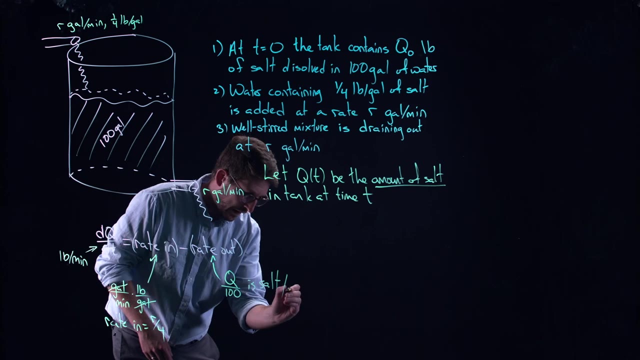 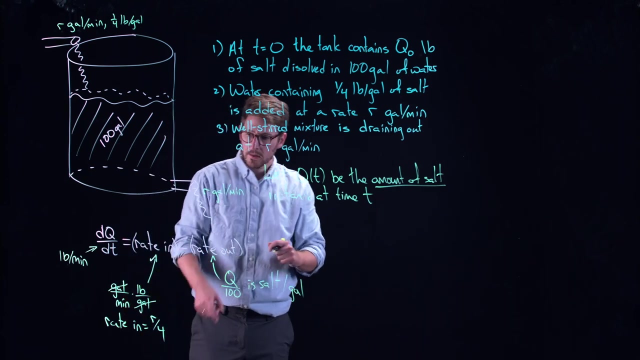 That tells you that if you have Q pounds of salt inside of this entire 100 gallons, then Q over 100 is salt per gallon. Sorry, pounds of salt per gallon. Okay, now I'm in a pounds per gallon situation And we know that. 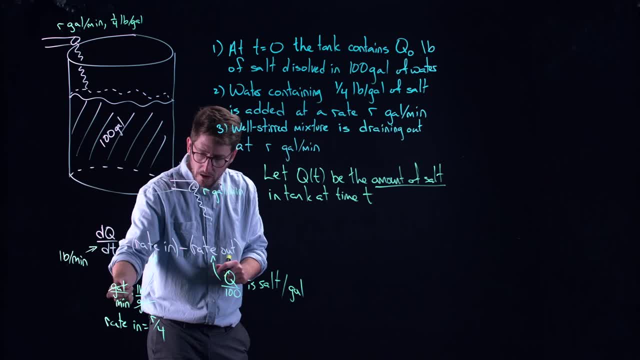 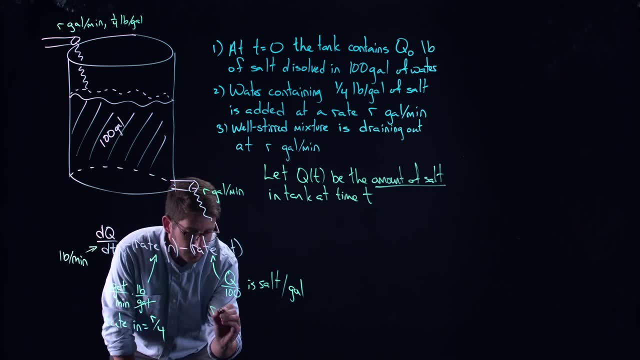 it's going out at exactly the same rate. So now that I've got pounds per gallon and I already knew the gallons per minute is the rate, Alright, sorry, it's r. This tells me that the rate out is equal to rq over 100.. Same thing. 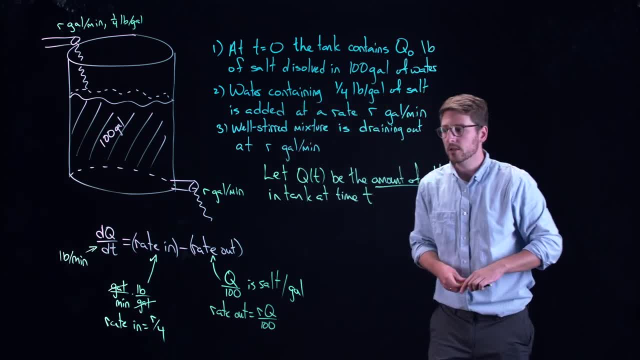 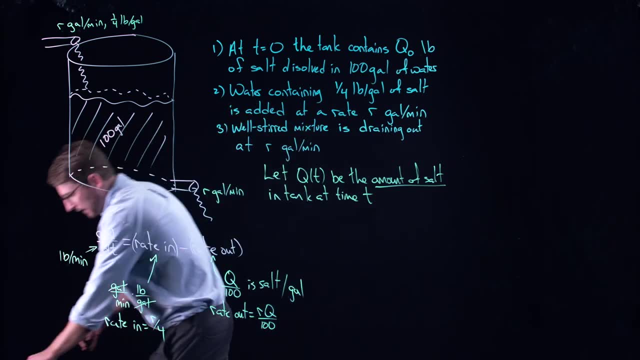 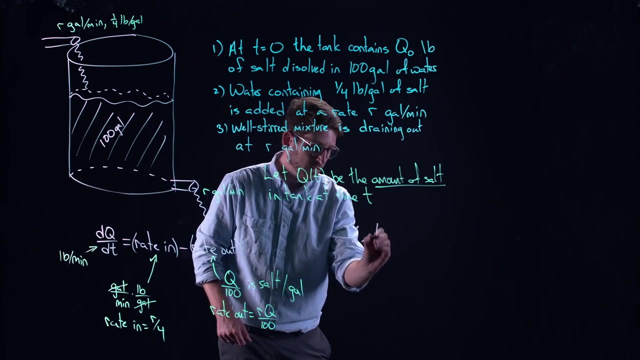 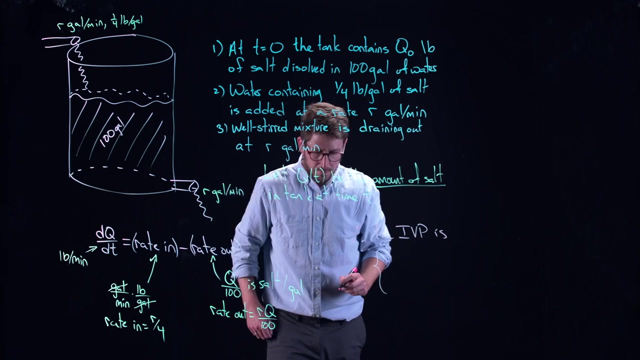 The only thing that I needed to know was how much, how many pounds per gallon of salt, I have inside the tank, And that means that I can put everything together here And I can say that, therefore, the IVP, the initial value problem, is the following: Well, I've got dq, dt rate, t, rq, rq, rq, rq, rq, rq, rq. 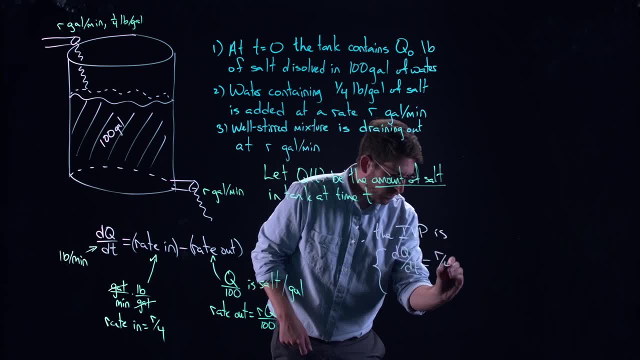 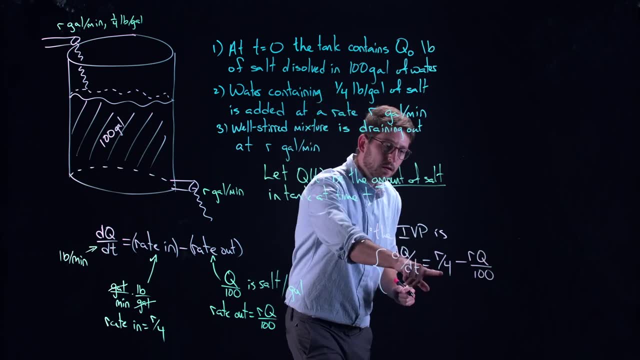 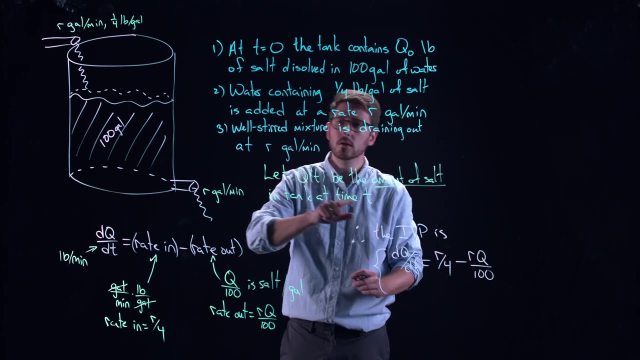 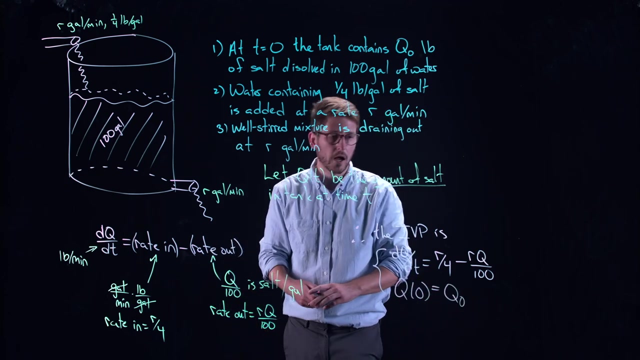 In minus, rate out r over four minus rq over 100.. Rate in minus rate out. That's what we just derived here. Remember I in IVP stands for initial, So our initial value is: q of zero is equal to q naught. 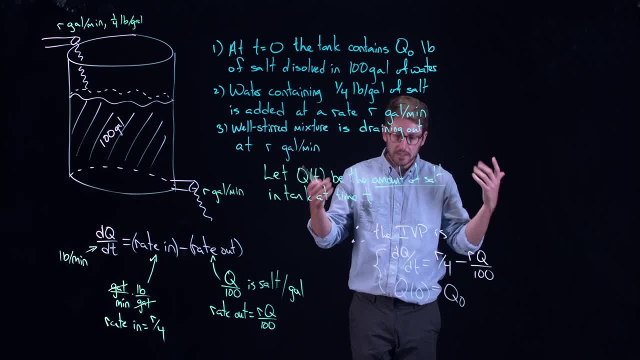 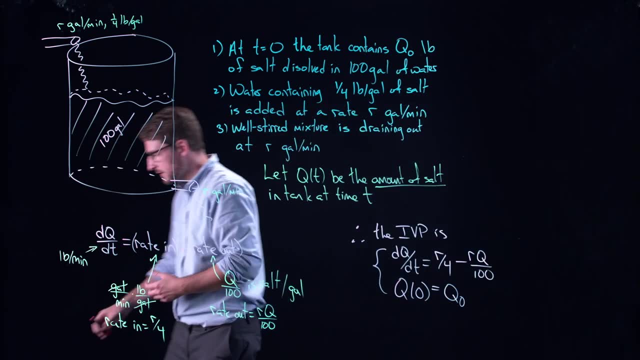 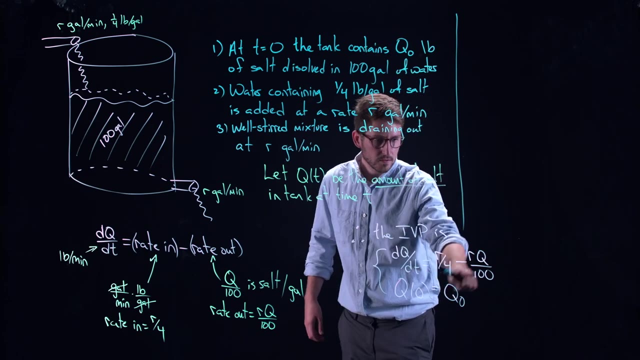 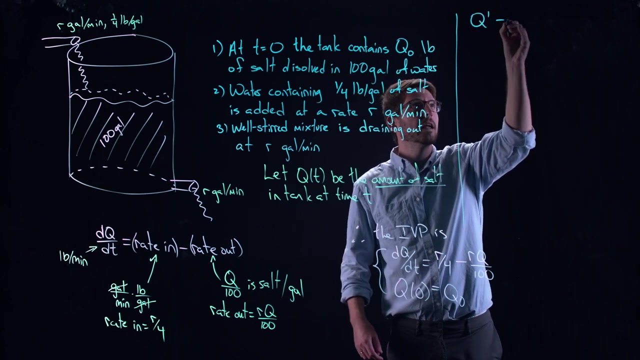 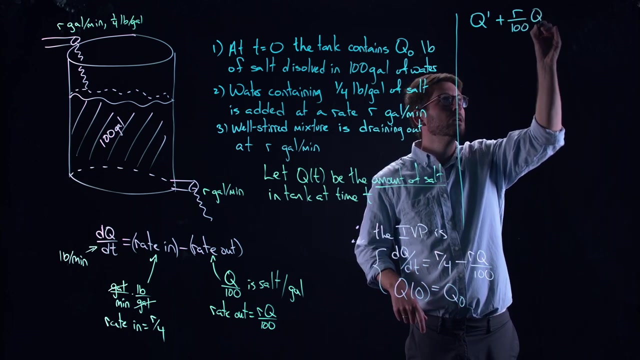 Nice, Easy peasy. right Now, what we have at our disposal is a way to actually solve this thing too, right, So let's go ahead and do it. So this differential equation, if I rewrite it, So let me write it as q prime minus, sorry, plus, once I pull this piece over: r over 100q is equal to r over 100. 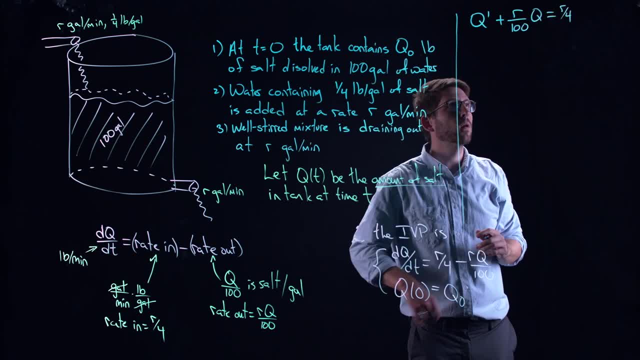 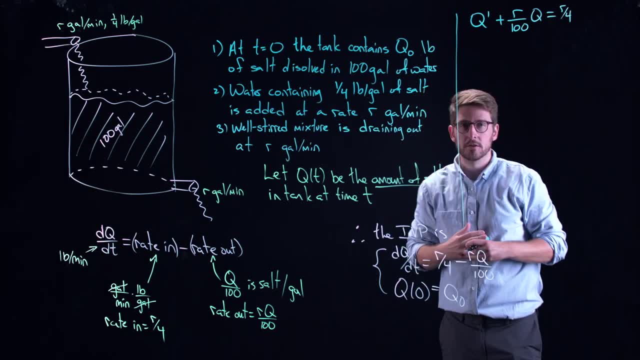 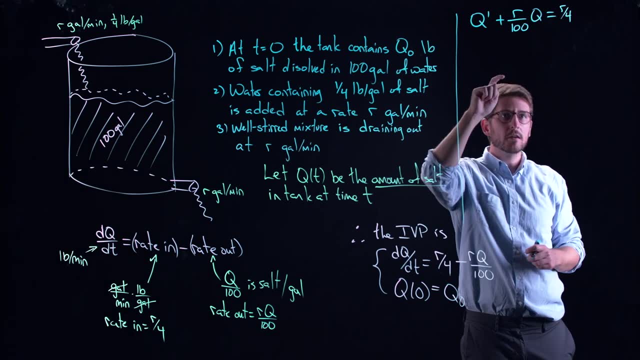 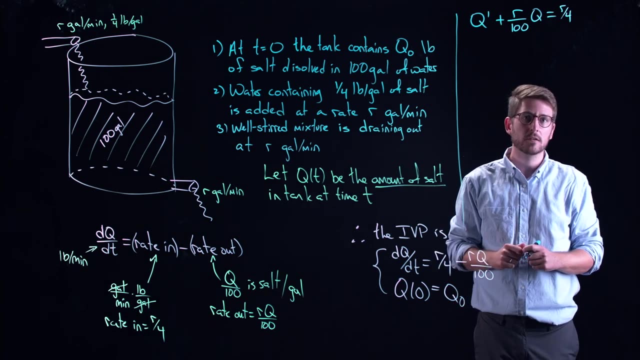 Why did I write it like that? Because I want a light bulb to turn on in your head And, in particular, I want you to say: ah, that is a first order linear, ordinary differential equation. And I know what to do with that type of equation because Jason told me two. 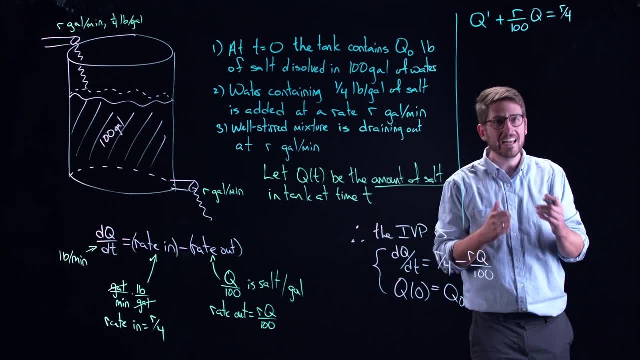 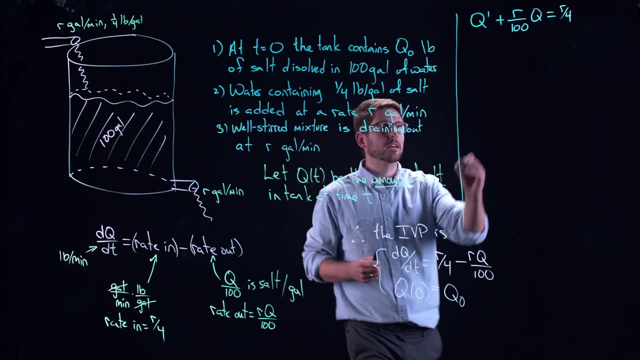 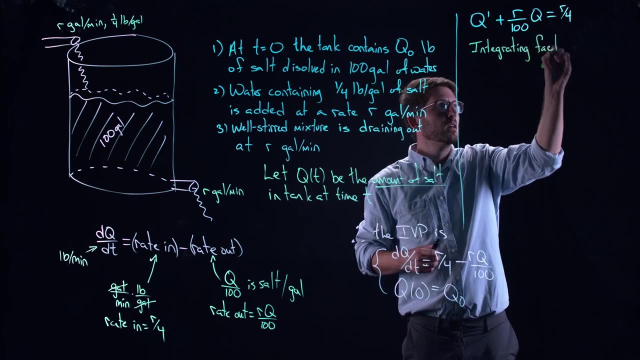 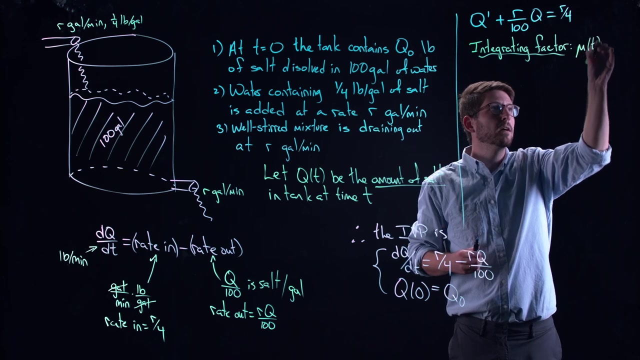 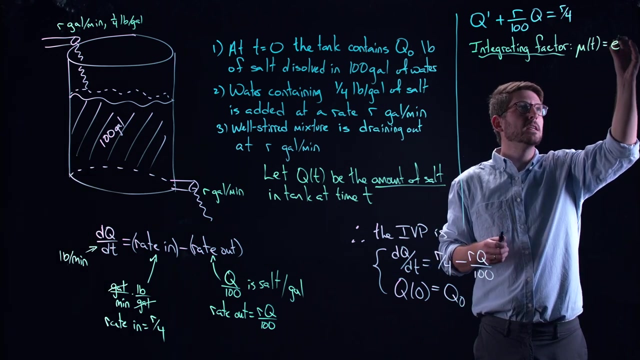 lectures ago. What he told me was that I need to use an integrating factor. OK, What he told me was that I need to use an integrating factor. OK, So let's do it. Our integrating factor, So integrating factor. Well, in our case, our p of t function is constant, So we remember how to do this. In this case, we called it a two videos ago, But in this case it becomes e to the r t over 100. 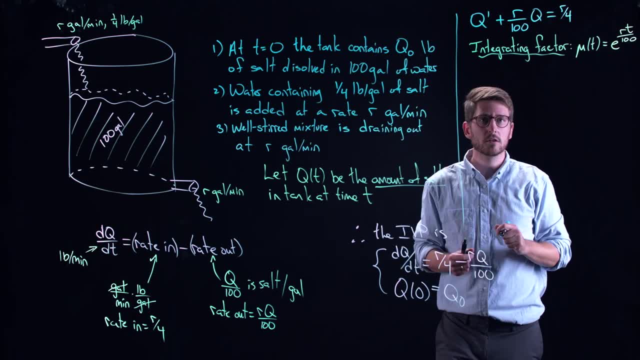 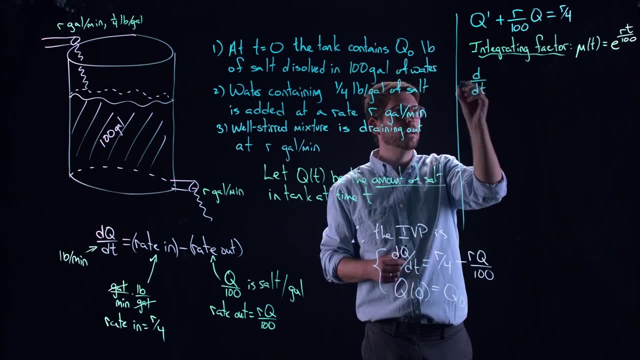 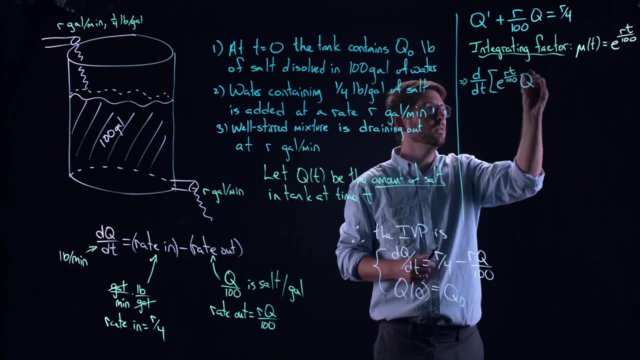 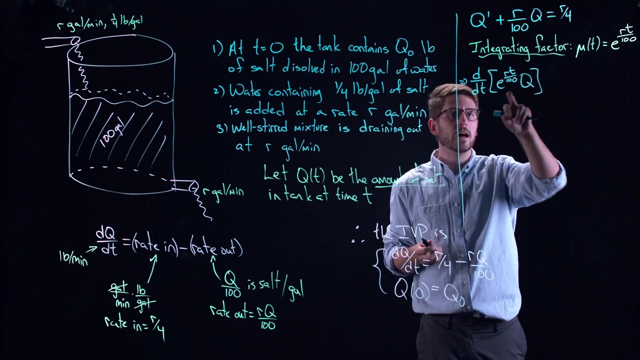 Okay. so then when you put that integrating factor into your equation, you multiply all three of these terms by mu of t. We know that by the choice of that integrating factor, I get e to the r, t over 100 times q, all taken with a derivative. Remember, that was the whole purpose of an integrating factor. The goal is to undo a product rule. 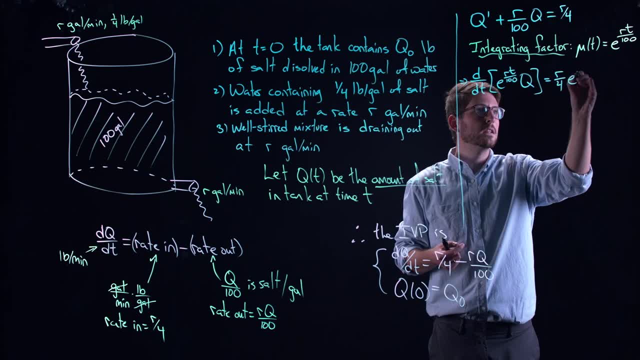 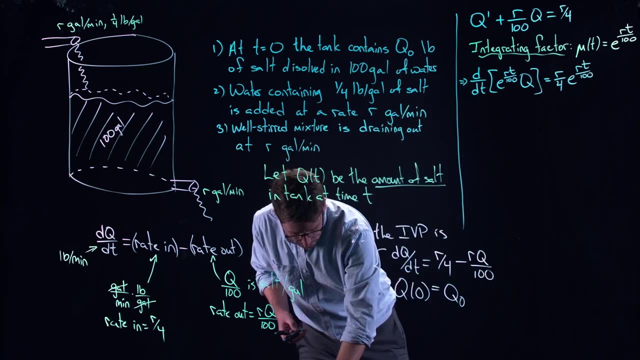 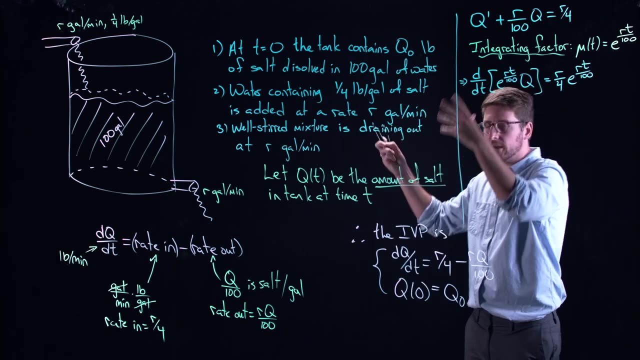 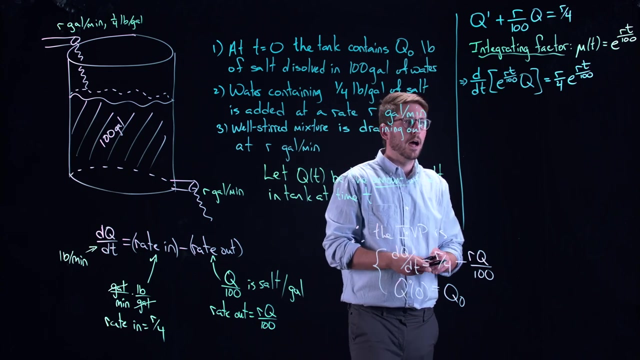 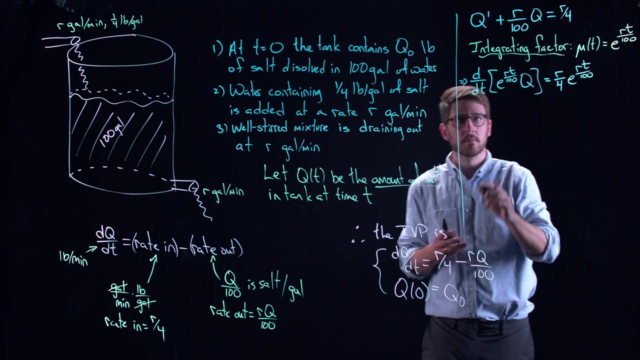 This leaves me with r over four, e to the r t over 100.. Okay, now remember, I gave you, I called it. I said like, in general, the procedure is that always, whenever we got to this point, I said: just integrate and solve, nothing left. It's too complicated, So I'm going to go ahead and just put the solution up, In this case, integrate it up, And then don't forget the, the constant here, and divide off this term. And so therefore, we can do this. 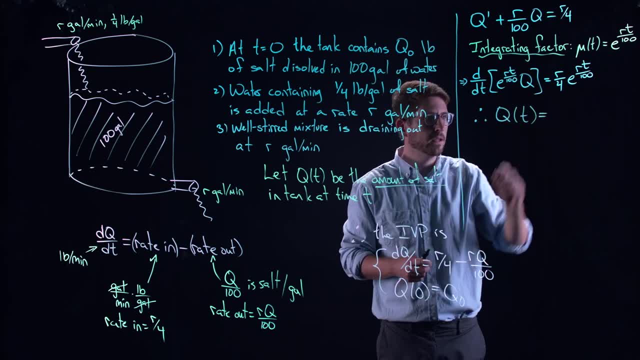 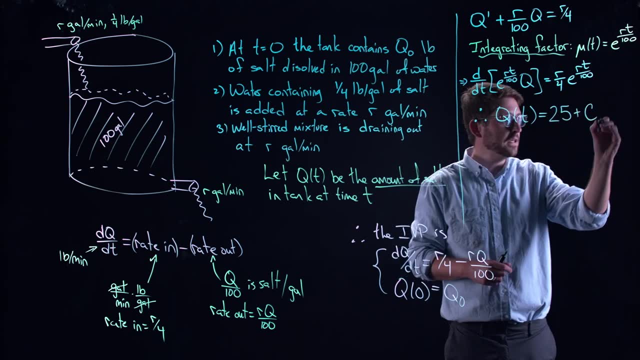 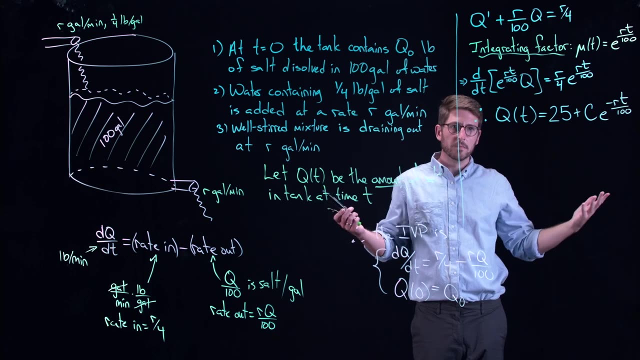 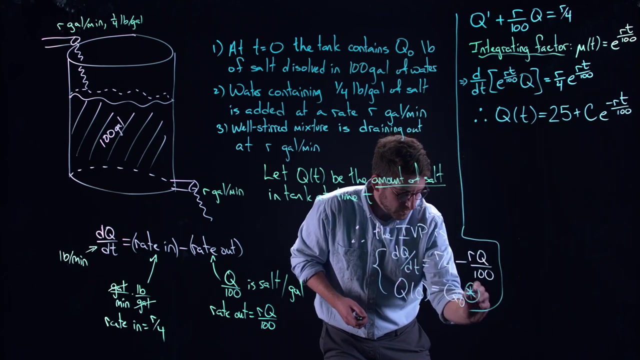 We get a general solution, q of t in this case, which is equal to 25 plus c, e, to the minus r t over 100.. Beautiful right, But we didn't quite solve it all. Notice that we have an initial condition as well. So also. 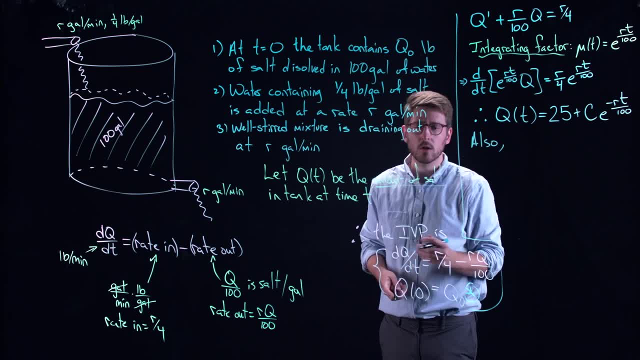 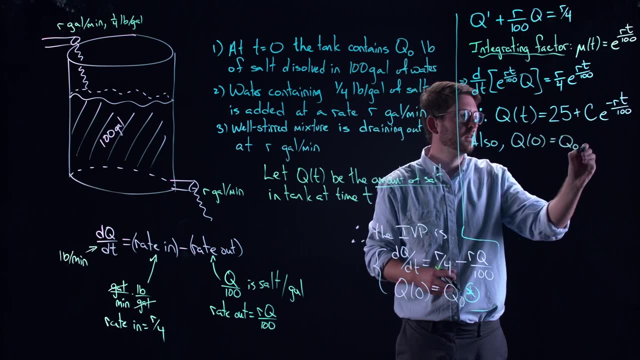 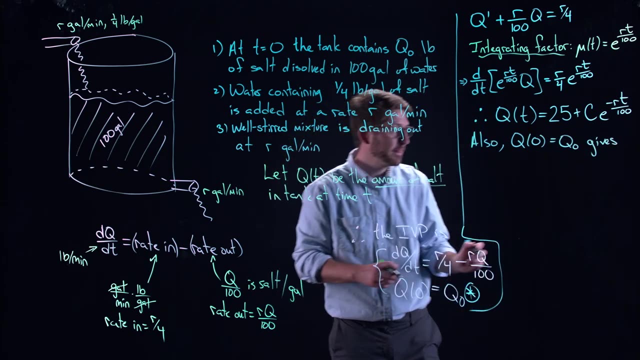 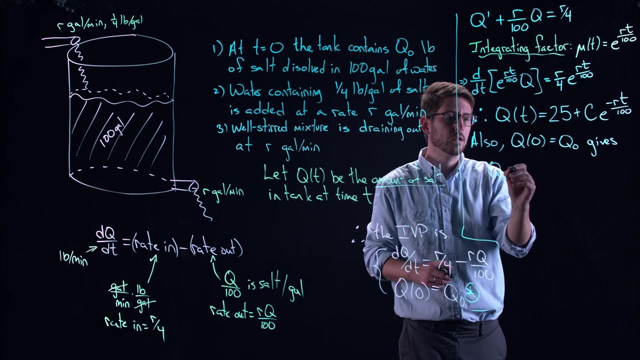 So I'm just kind of putting it in here because there's not a whole lot left to talk about it for this. But also: q of zero is equal to q naught gives. well, this is going to pin down a value of c. So in this case I get q naught. when I put t equal to zero in here, I get q of zero, which is q naught. this becomes 25 plus c. e to the minus r, t over 100. 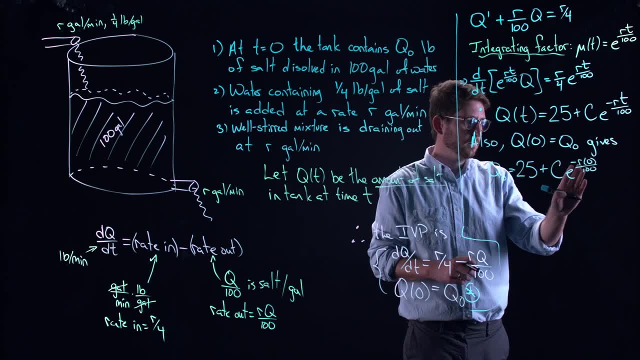 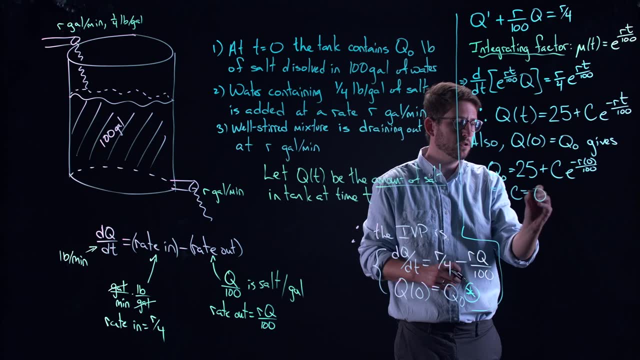 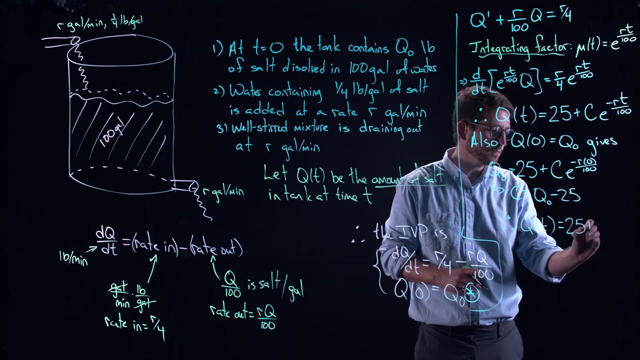 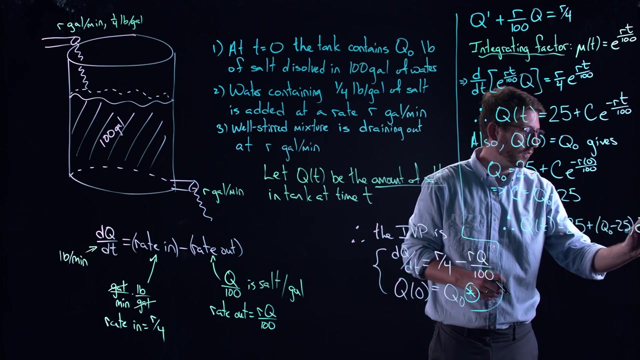 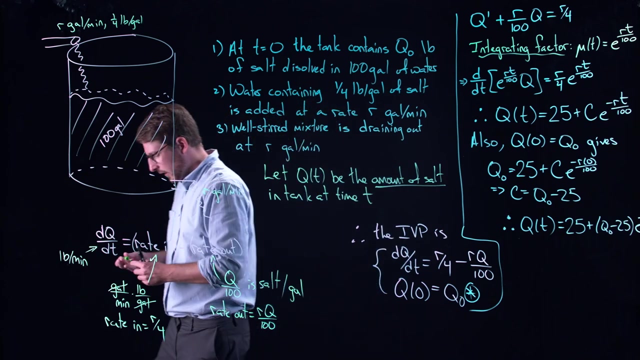 r times 0 over 100.. This whole thing becomes 1, and that tells me that c is equal to q naught minus 25.. And so, therefore, now I have a solution, a particular solution, to my initial value problem, which is 25 plus q naught minus 25, e to the minus rt over 100.. Okay, before we conclude this video, 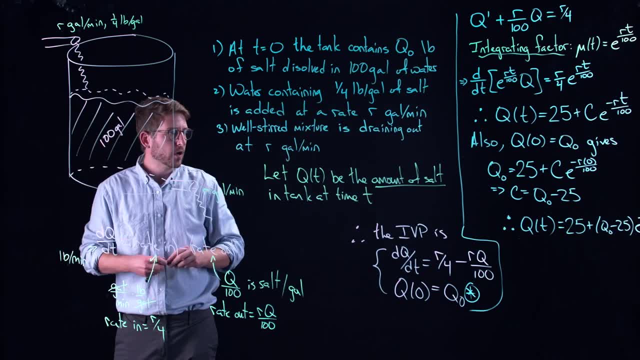 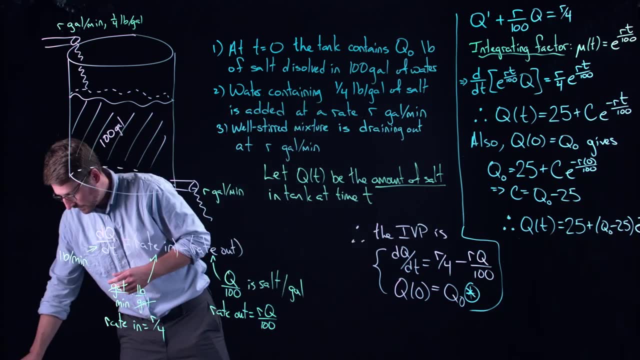 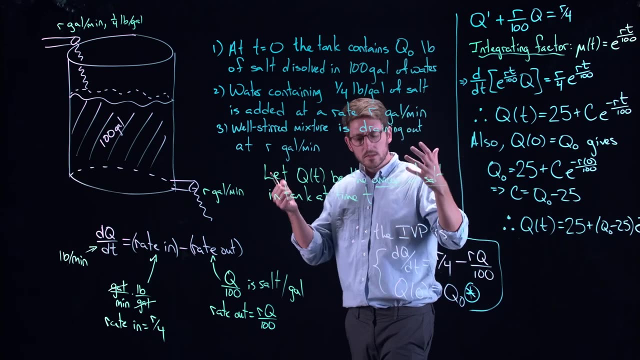 I want to discuss what is going on with this solution, right? So there's some things that I can easily identify that are important for this equation, The first of which is this: value 25.. 25, that sort of, keeps coming up. What does 25 represent? Well, again, pause the video and see. 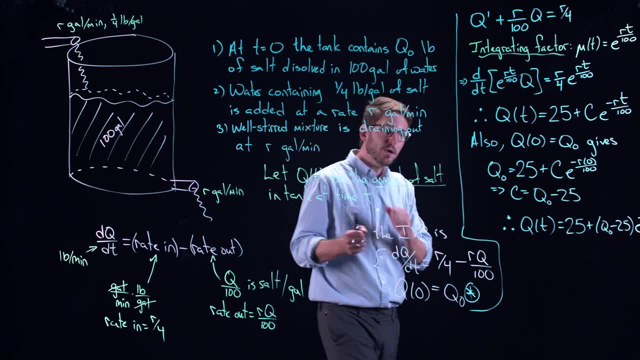 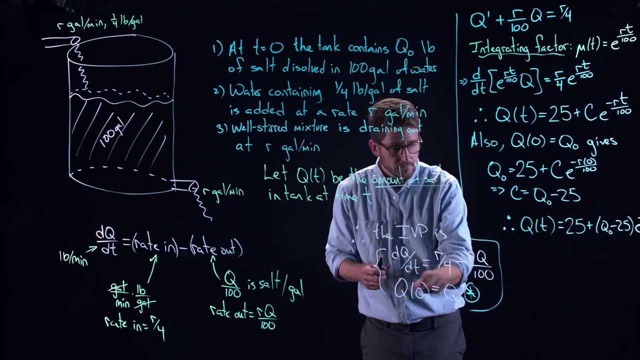 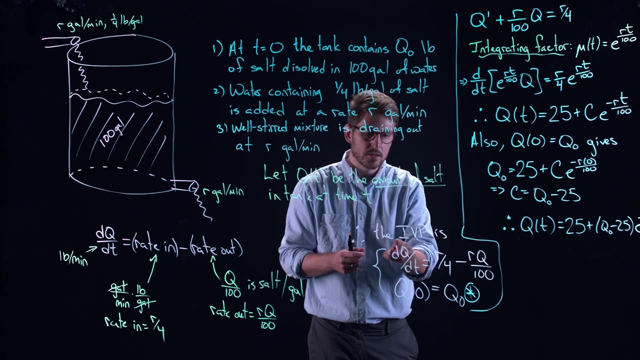 if you can figure it out for yourself, But if you didn't pause the video and you would like me to tell you that 25 represents the equilibrium value of my differential equation, Look it, Remember. the equilibrium is when the derivative is equal to 0, dq by dt. 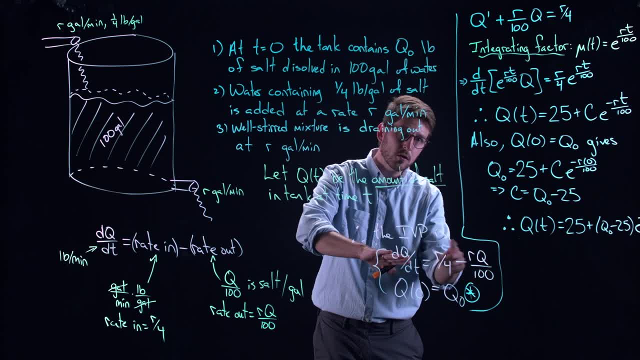 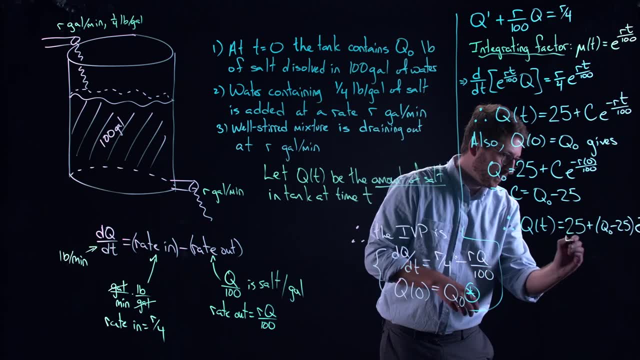 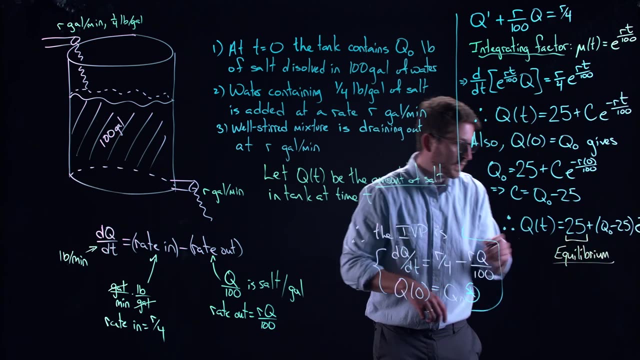 that's equal to 0.. I've got a linear equation that I need to solve for q, which you can very easily find q to be 25.. So this is the equilibrium. So something that we talked about in the very first video is coming back Then. 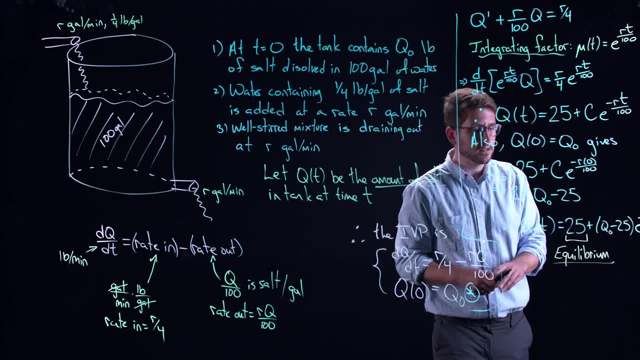 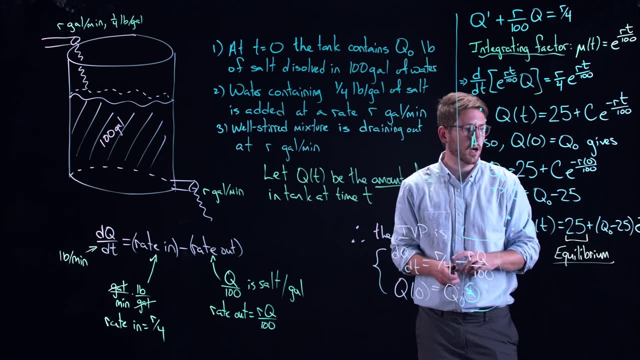 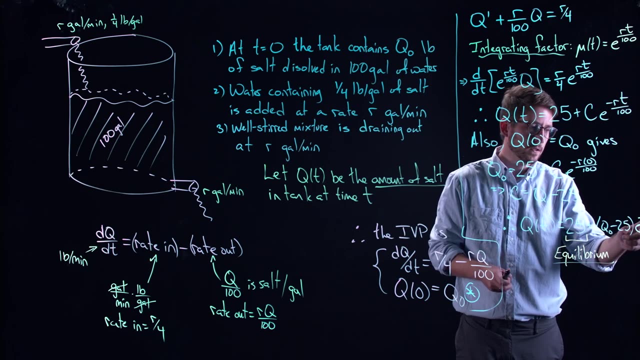 let's look at the other components of this differential equation, the part that's changing in time. What's happening? So this partner that's creating the curve here, this frequent infection caught up with this part of the del Q, has a tidal change in time here as time goes on. 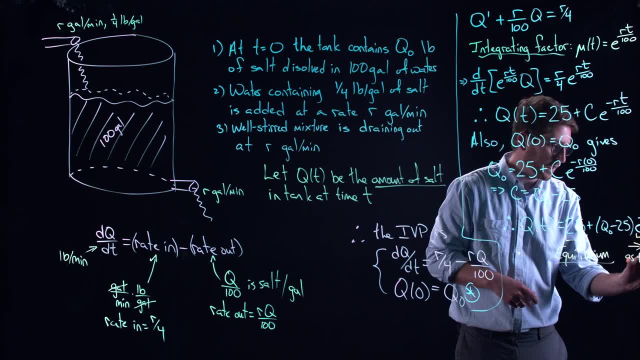 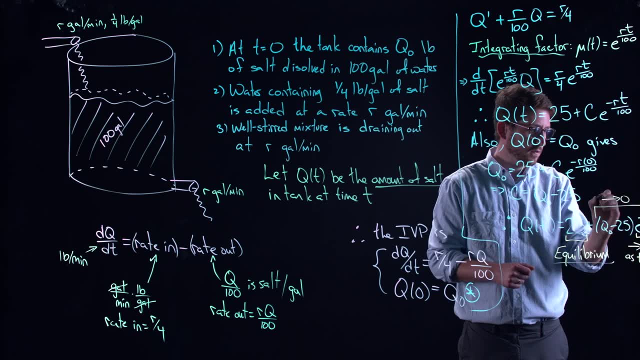 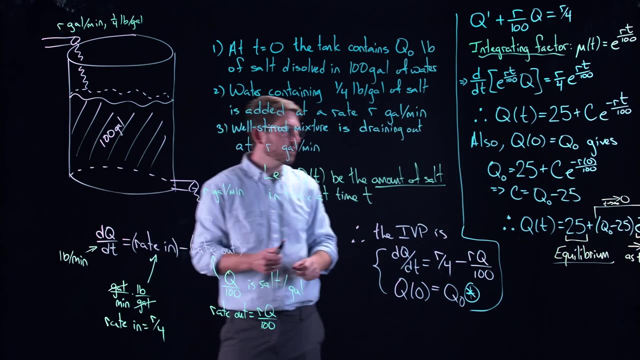 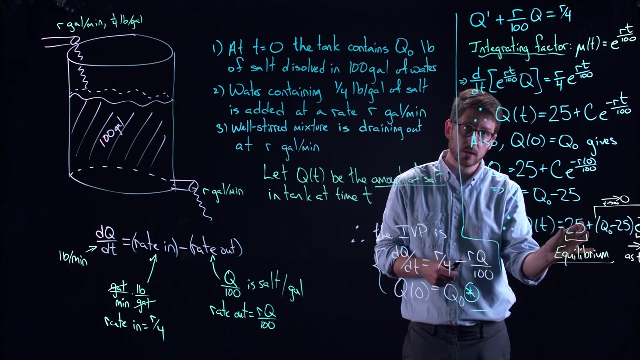 well, as time goes to infinity, since we're going to assume, of course, that R is positive, this piece right here, this goes to zero. as time goes to infinity, This piece is decaying, Which means that the whole thing? Well, it tells you that, no matter how you start with Q naught, you always will settle into the equilibrium. 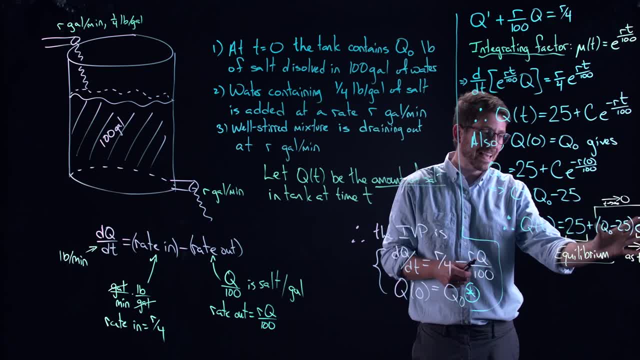 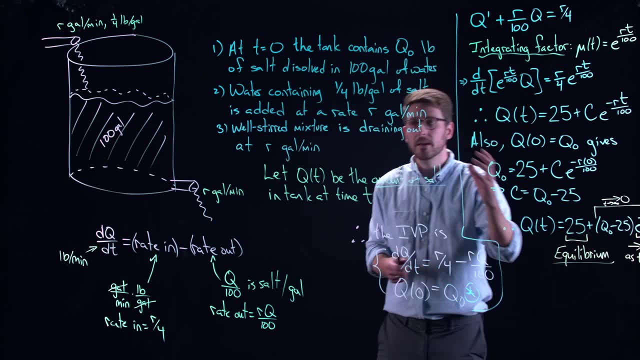 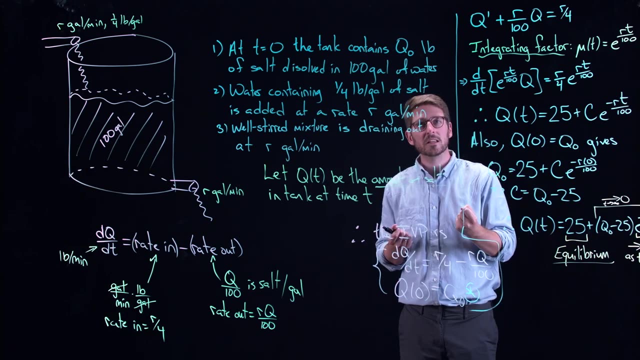 That comes from the fact that this piece right here is decaying in time. It's disappearing, leaving you with just the equilibrium value. This should feel very, very, very familiar, right? Because this is the exact same thing that we saw happen in the very first lecture with the motion of a falling object. 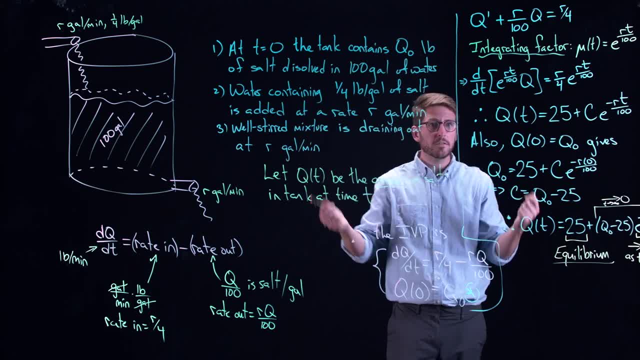 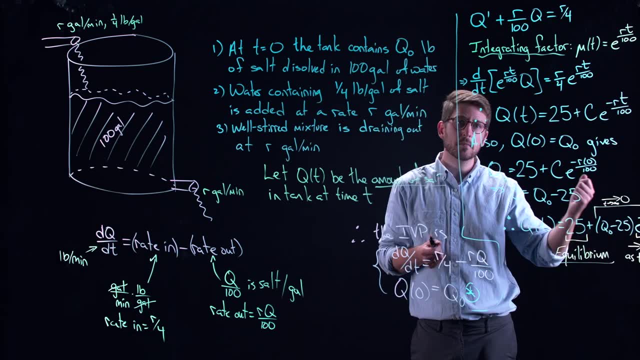 Now these are two physically very, very different scenarios, But if you go back and compare with the solution from the motion of the falling object, it's very, very, very similar. In fact we saw again with that case that everything settles into the equilibrium. 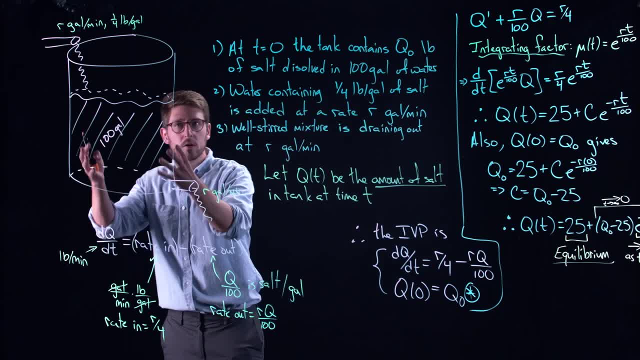 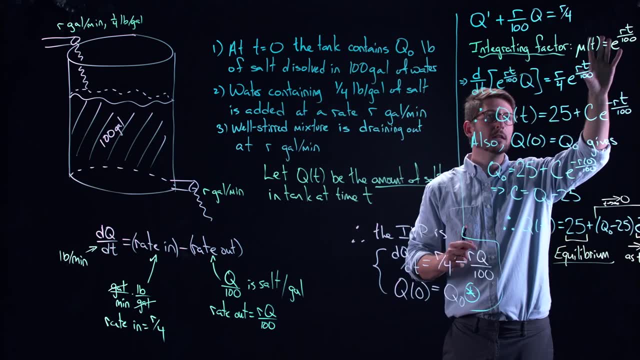 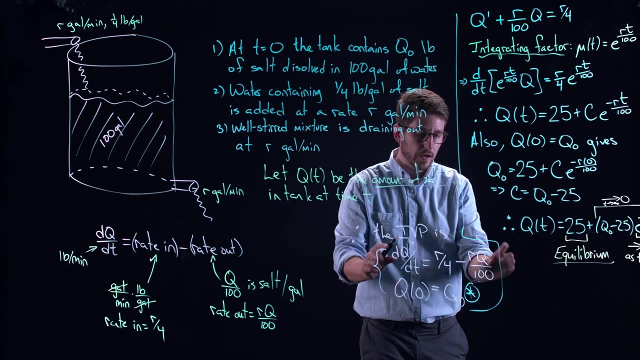 So, even though we derived an equation for this sort of chemical problem, we got something that looked very similar And we got to show off with a new shiny tool of the integrating factor. We got to see how that thing can work. If you want to solve this thing as a separable equation, that's perfectly acceptable. 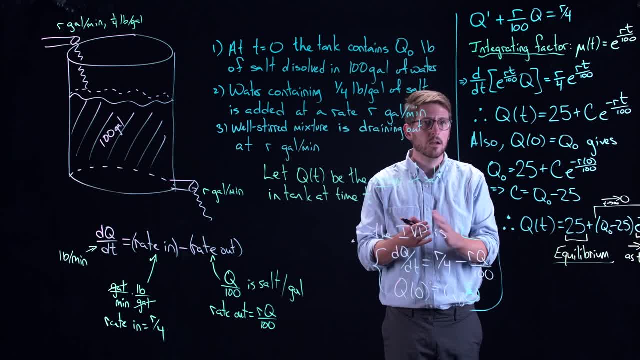 You could do that as well. If you would like to see how to do that, just go back to the first lecture and take a look at what we did with the motion of the falling object.